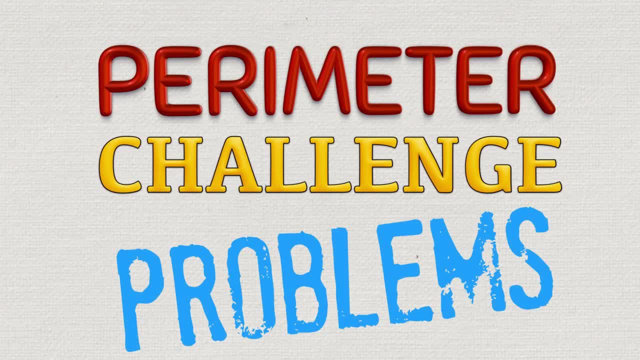 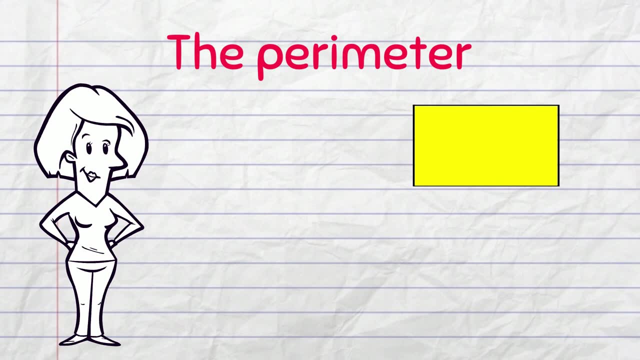 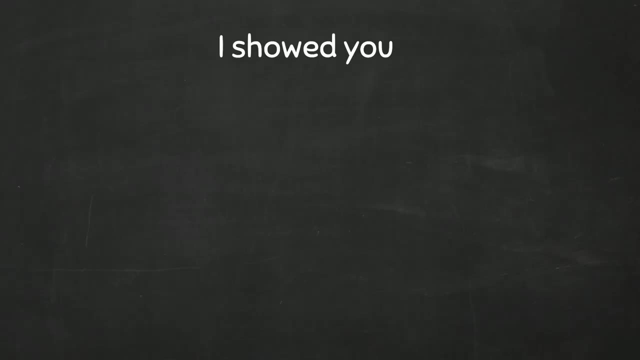 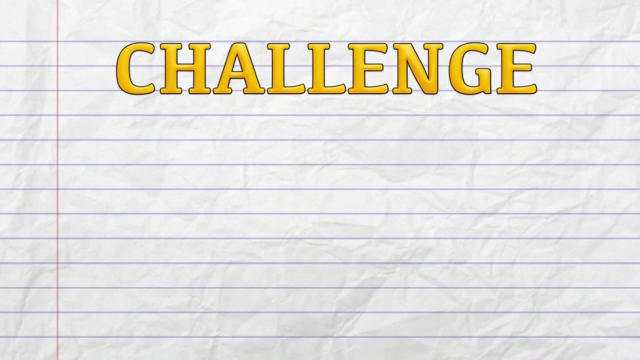 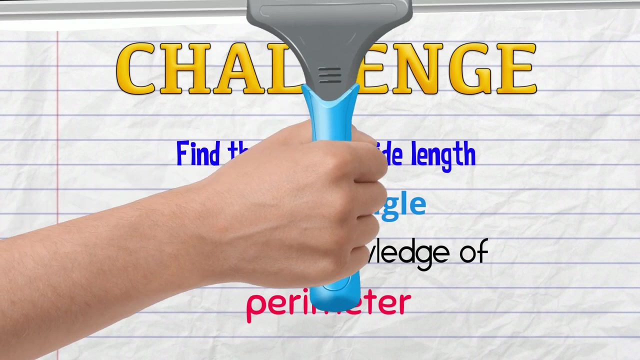 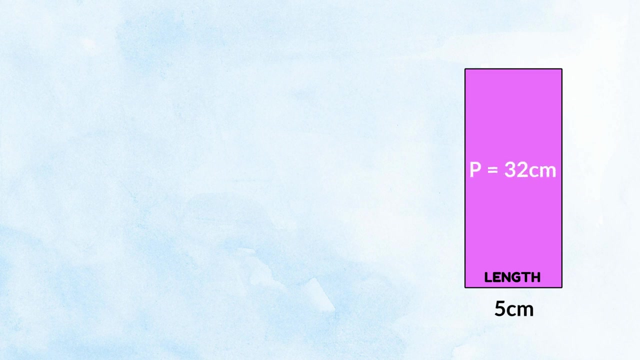 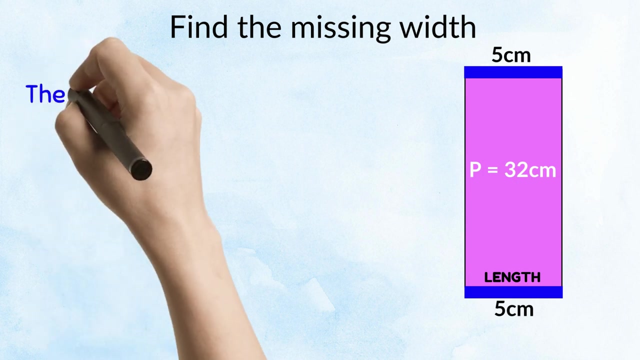 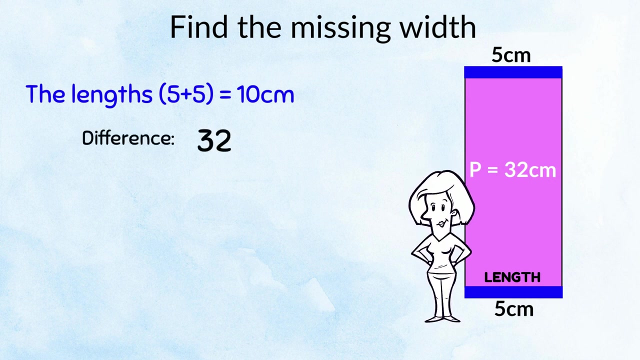 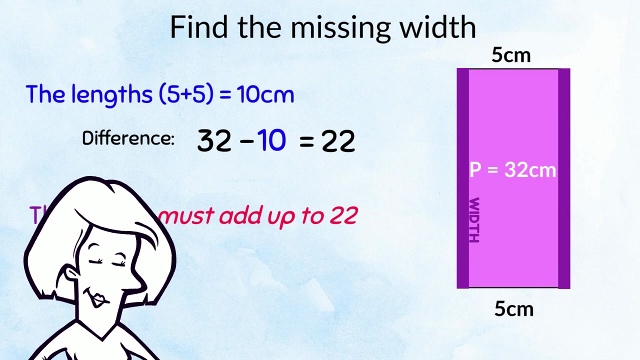 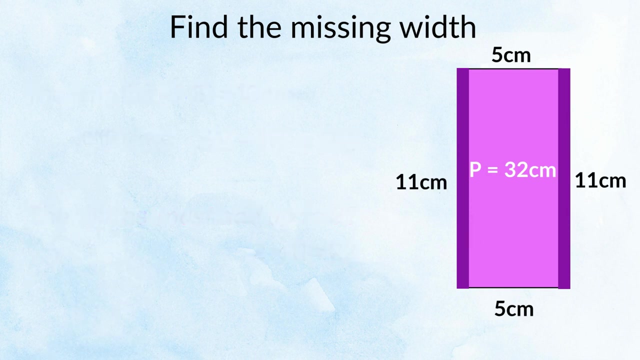 PERIMETER CHALLENGE PROBLEMS. PERIMETER 12 x 22. If you know your tables, you'll spot that 2 x 11 is 22, so the missing width is 11cm. We can add up the sides. 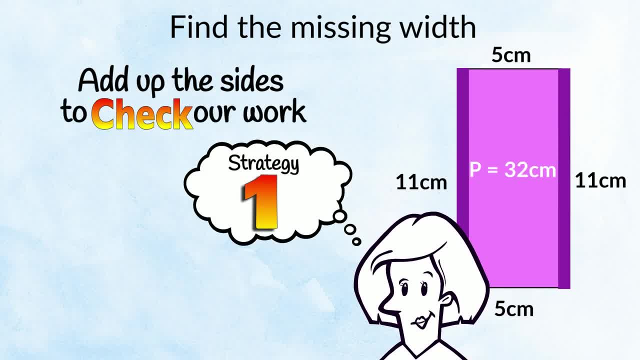 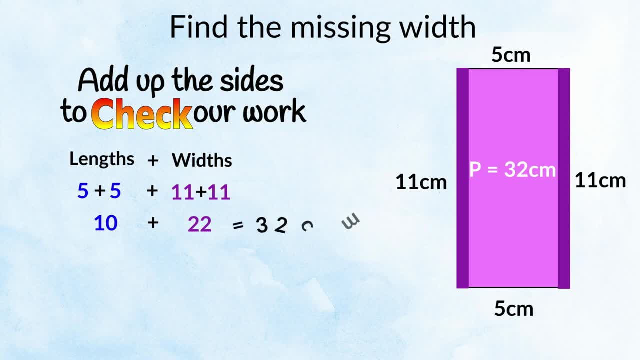 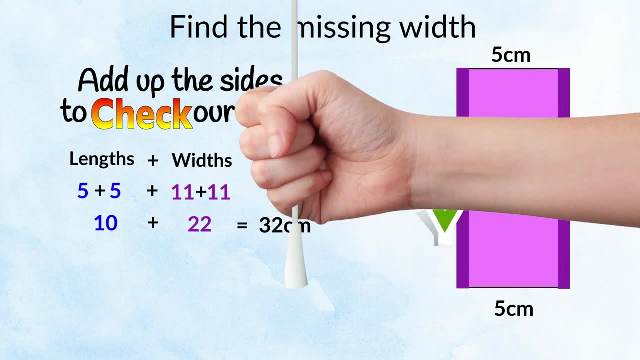 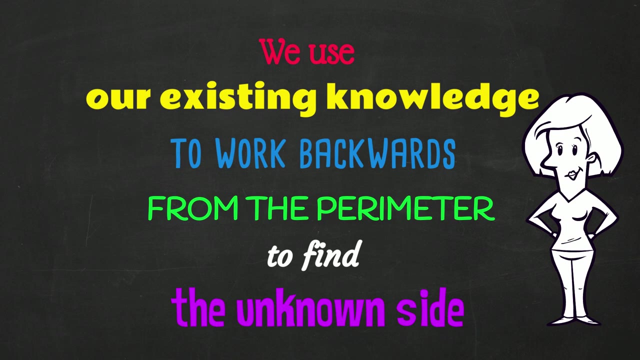 to check our work: The length plus the width, 10 plus 22, that's 32. So we're right. The missing width is 11cm. See, We use our existing knowledge to work backwards from the perimeter to find the unknown side. 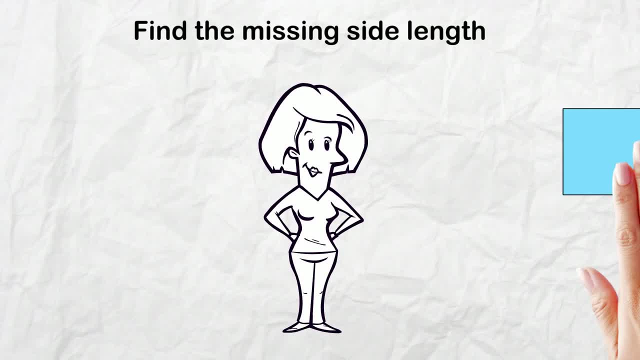 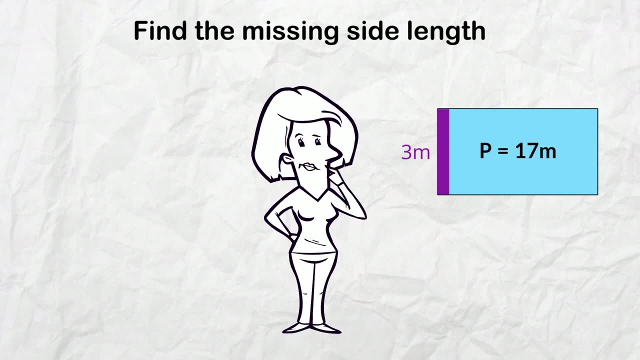 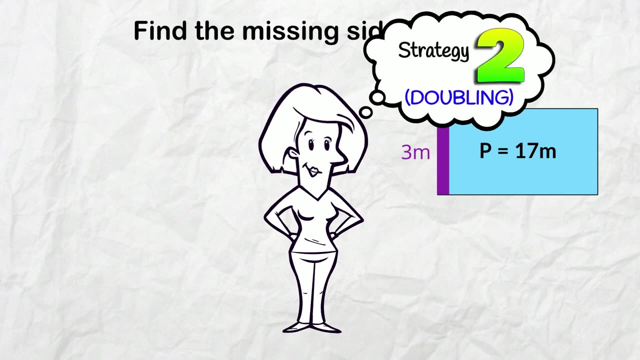 Cool, Let's do another one. Here's our rectangle: The width is 3m and the perimeter is 17- An odd number. This time I'm going to use Strategy number 2, The doubling strategy. The width is 3, Double 3 is 6. 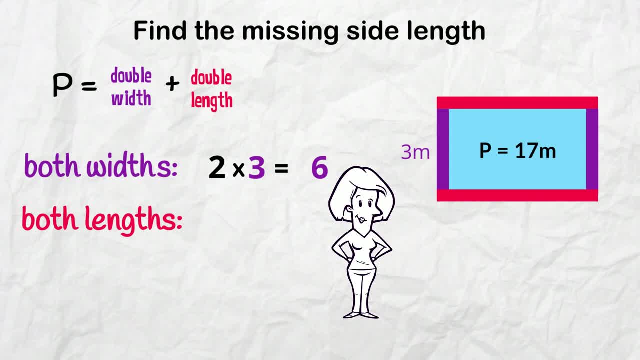 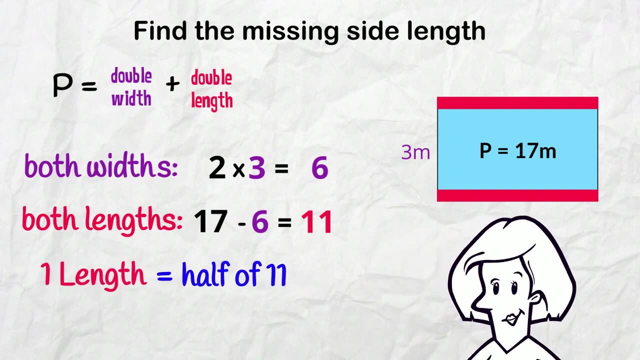 Now for these lengths. We think perimeter minus the doubled width, So 17 minus 6, That gives us 11. One length is half of 11, So 11 divided by 2- I know there's going to be a remainder of 1 because 11 is an odd number. 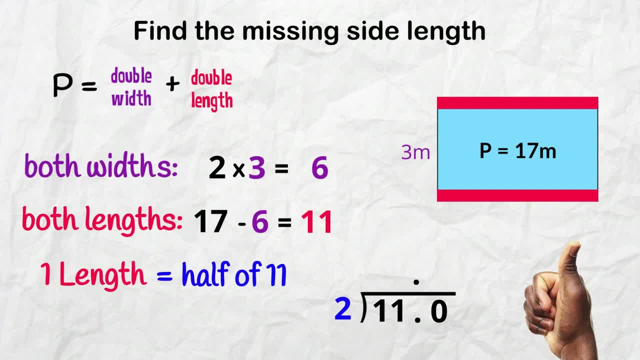 I set it up for a decimal remainder because that's the best way to show a measurement, Alright, 2 x 11, 5 x 2 is 10, Remainder 1. Now, 2 x 10, 5, 11 divided by 2 is 5.5.